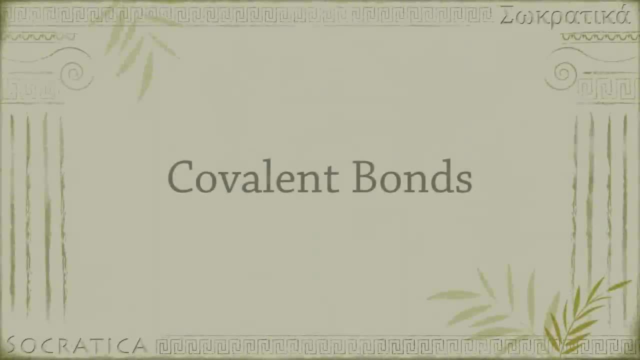 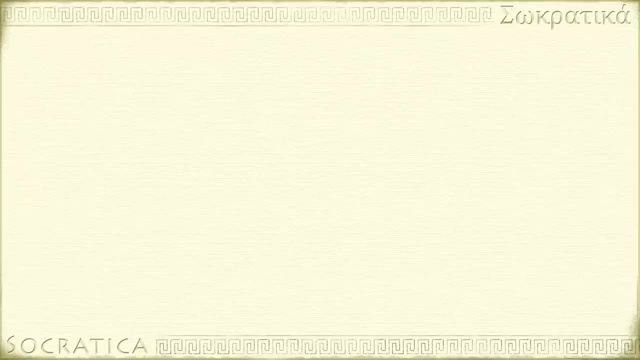 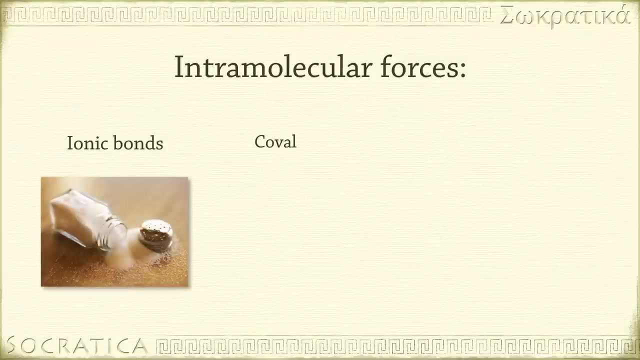 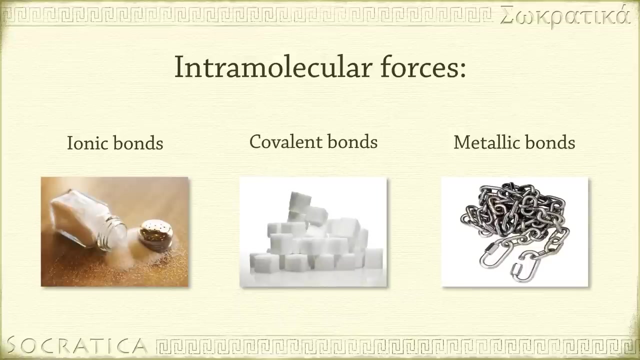 The bonds that hold atoms together in compounds are called intramolecular forces. The three main types of intramolecular forces are ionic bonds, covalent bonds and metallic bonds. This video will focus on covalent bonds. Ionic bonds and metallic bonds will be featured in their own. 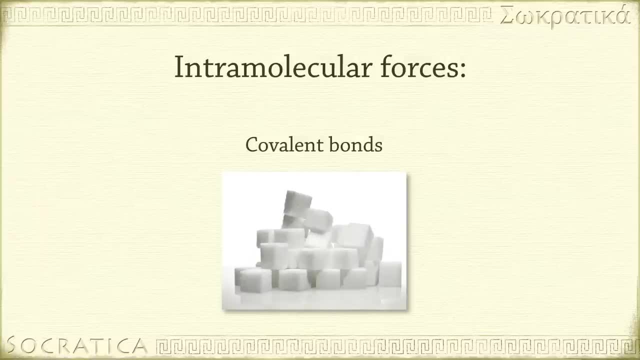 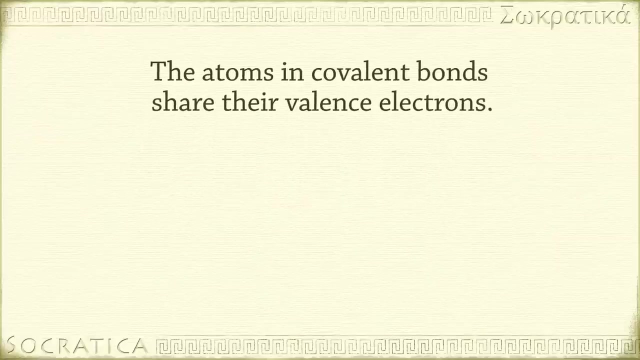 videos. Covalent bonds are stable because the bonding atoms achieve noble gas configuration by sharing electrons. The name covalent should suggest to you that the atoms are sharing their valence electrons. We can show this with a Lewis dot diagram: Hydrogen, fluoride, HF. 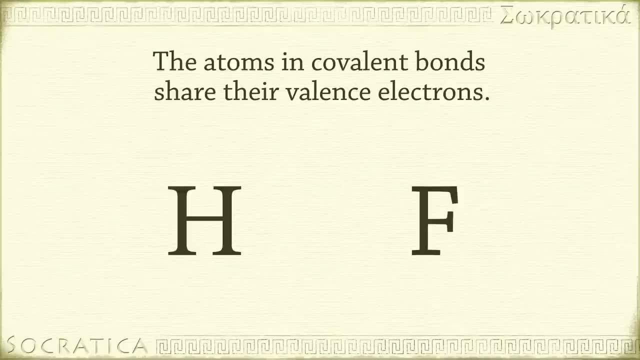 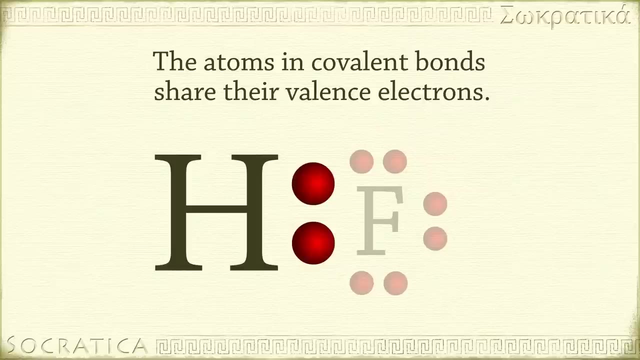 is a molecule with a single covalent bond formed between two atoms. Fluorine has seven valence electrons and hydrogen has one By sharing two electrons in a bond. now hydrogen has two valence electrons and has the same electron configuration as the noble gas helium. Fluorine now has eight. 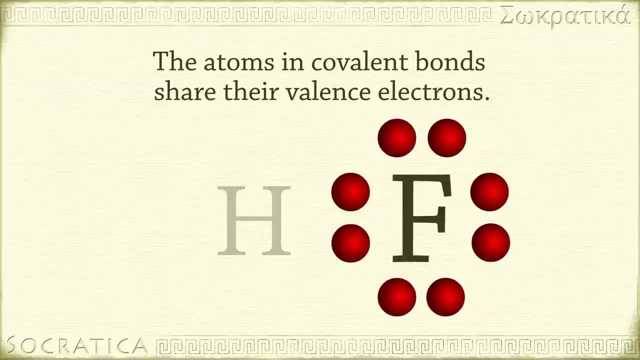 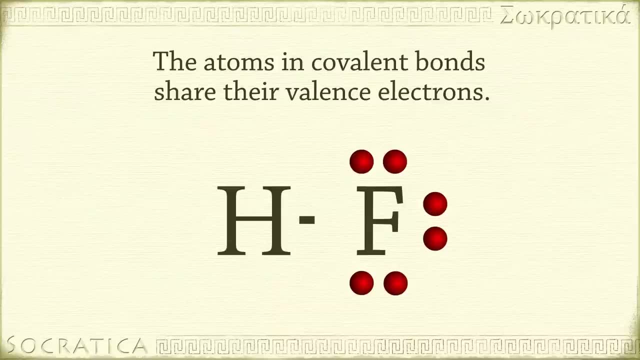 valence electrons and has the same electron configuration as the noble gas neon. We can replace those two shared electrons in the diagram by a single line representing the single covalent bond. Sometimes two atoms share more than two electrons in the case of a double or triple covalent bond. 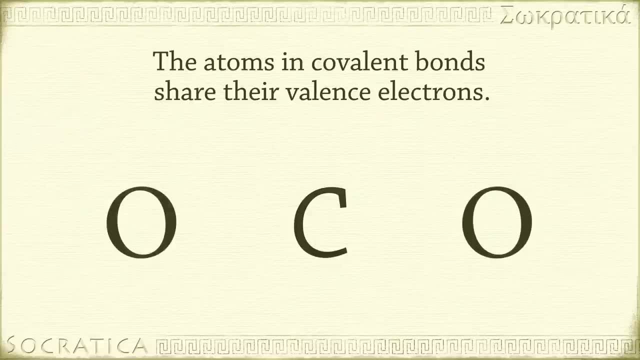 We can see an example of that in carbon dioxide, CO2.. The Lewis dot structure looks like this: Carbon has four valence electrons and oxygen has six valence electrons. Carbon needs four more electrons to achieve noble gas configuration. Oxygen needs two more electrons to achieve noble. 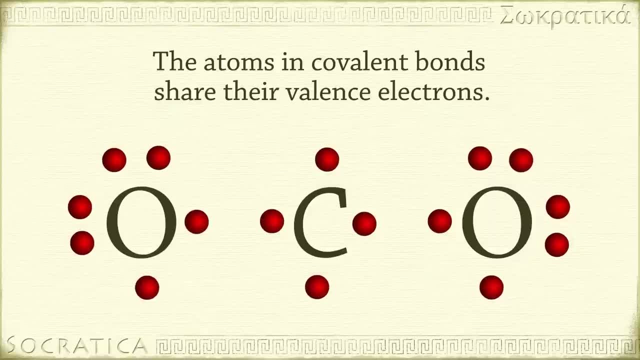 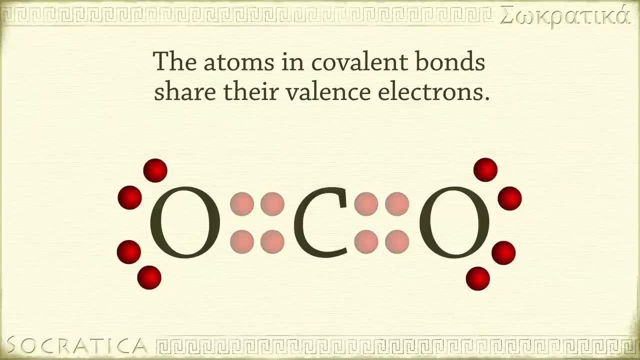 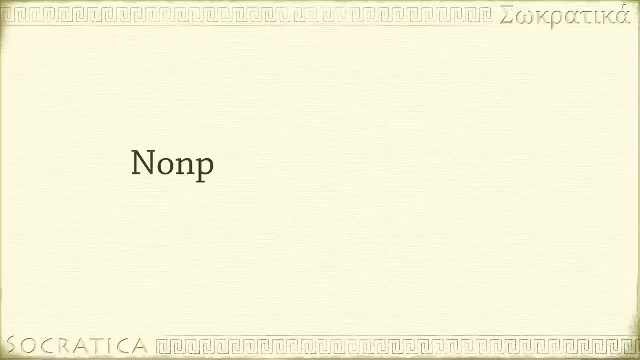 gas configuration. This can be achieved if the carbon atom forms two double bonds. with each oxygen atom, We can replace the two shared pairs of electrons in the diagram with two straight lines representing a double bond. If the two atoms in a covalent bond are identical, they have the exact same electronegativity as each other. Click here to learn more about electronegativity. 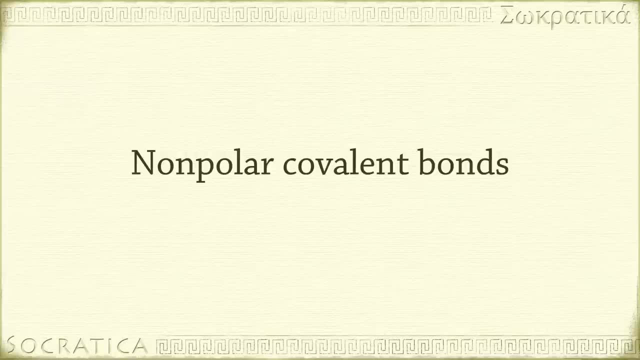 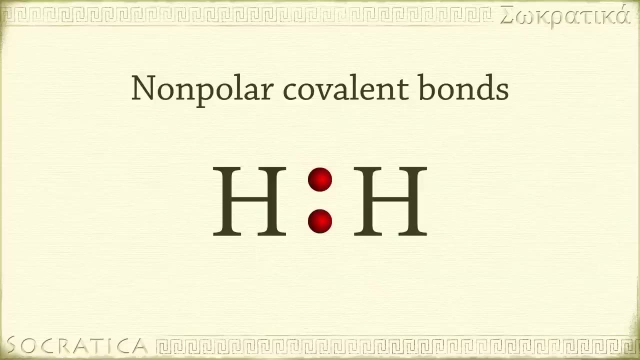 Click here to learn more about electronegativity. Click here to learn more about electronegativity. identical atoms is called a nonpolar covalent bond. Hydrogen, for instance, exists in nature as a diatomic molecule, H2.. 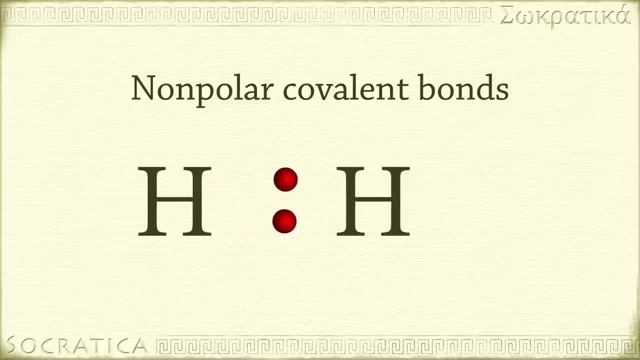 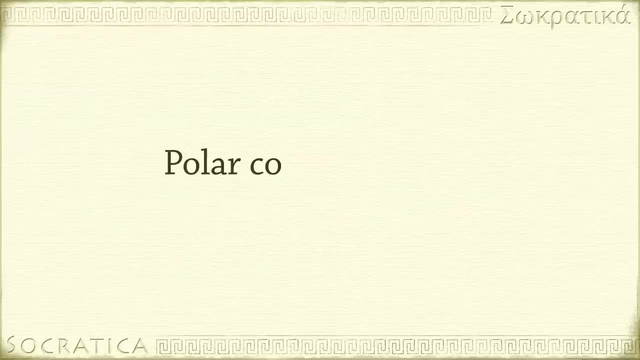 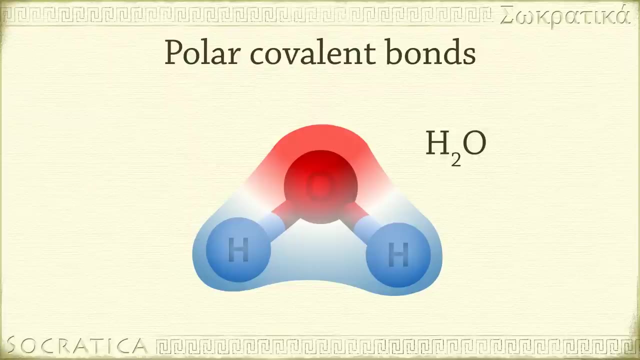 The two hydrogen atoms pull equally on the shared pair of electrons in the bond, so there is no directionality or polarity of the bond. Compare that with the bonds in a polar molecule like water. H2O Oxygen is much more electronegative than hydrogen. 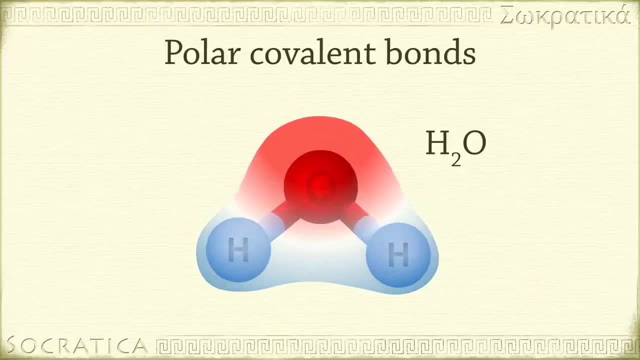 so the electrons in the covalent bonds spend more time around the oxygen than around the hydrogen. We call this kind of uneven sharing of electrons a polar covalent bond. Notice that this results in the water molecule being polar as a whole. One side of the molecule is more negative than the other side. 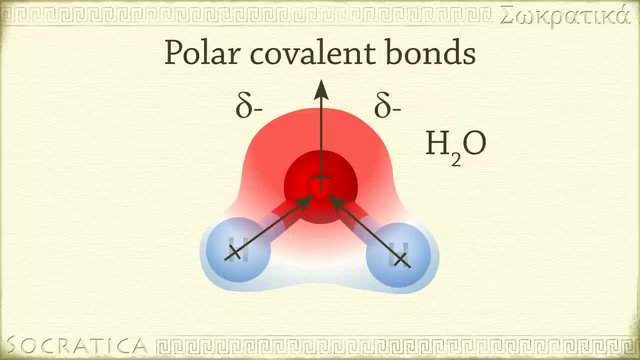 A lowercase delta is used to show the partial negative charge on the oxygen atom And the partial positive charge on the hydrogen atoms. We use this delta notation to distinguish these partial charges from the full charges carried by ions. You might get confused between molecules which contain polar covalent bonds and molecules. 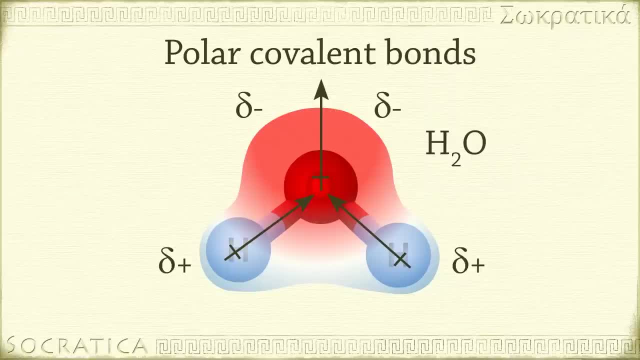 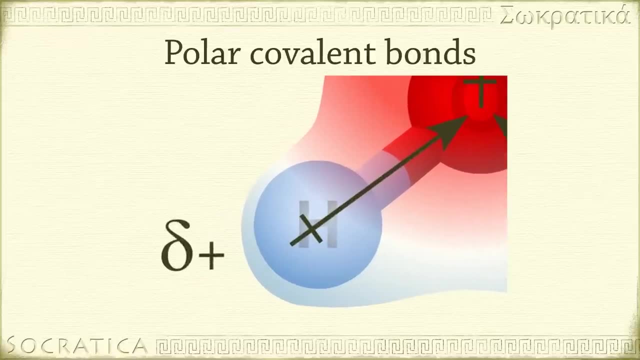 which are polar as a whole. Water is both. It contains polar bonds and is a polar molecule as a whole, because one end of the molecule is slightly positive and the other end is slightly positive, And the other end is slightly positive and the other side is slightly negative. 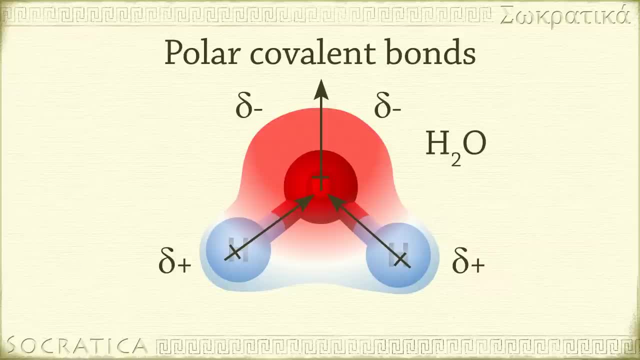 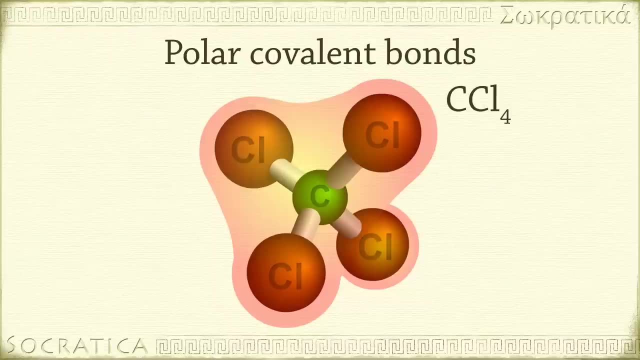 That's a result of the polar covalent bonds that hold the water molecule together. But consider the carbon tetrachloride molecule, CCL4.. Chlorine is more electronegative than carbon, so this molecule has four polar covalent bonds. 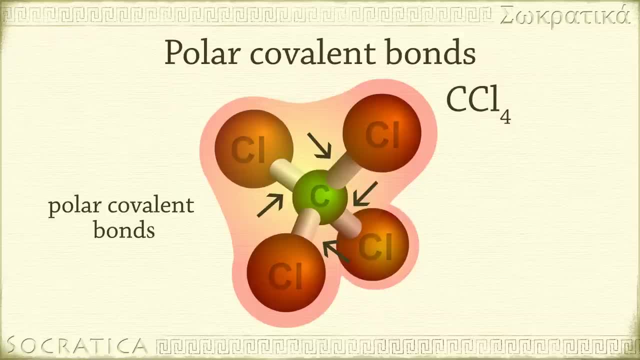 You might think, adding the four bonds together, this molecule is going to be very polar as a result, But actually, when you look at the three-dimensional structure, you see that the four bonds point in four opposite directions, so they cancel each other out. 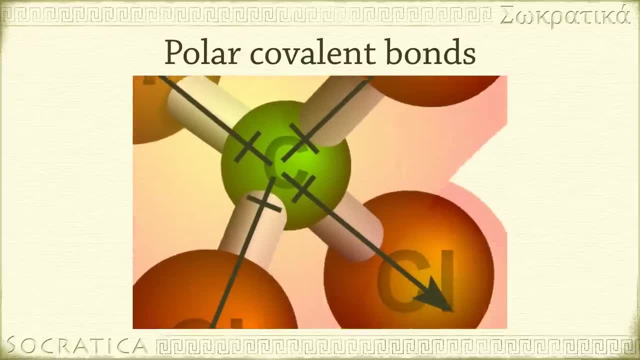 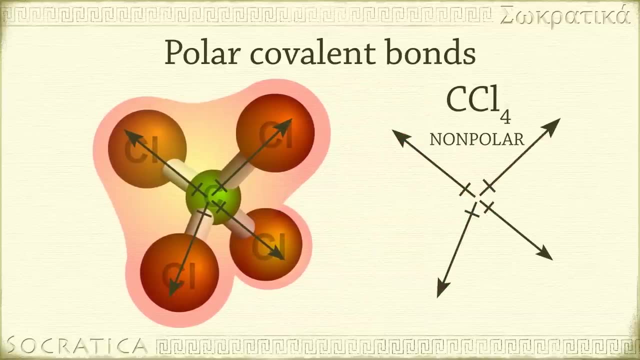 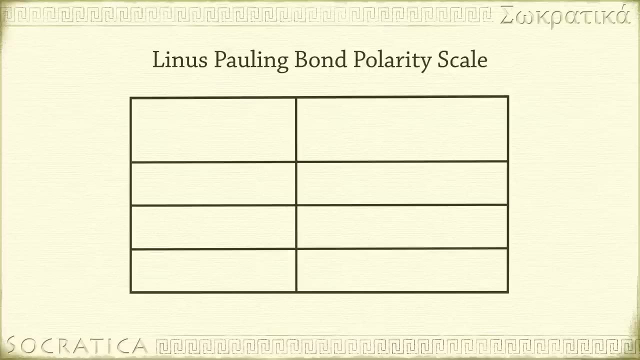 You can't find one side of CCL4 that is more negative or positive than the other, so carbon tetrachloride as a whole is a non-polar molecule. Chemists generally measure the polarity of a bond according to a scale established by Linus Pauling.